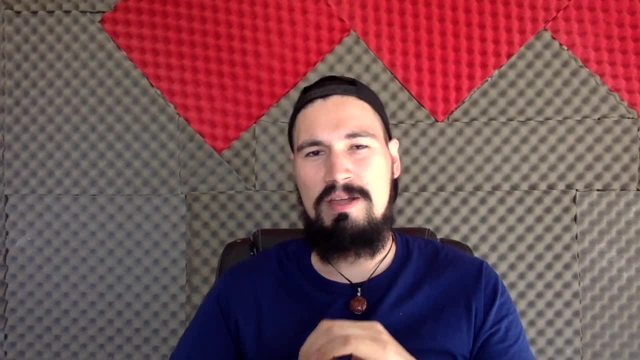 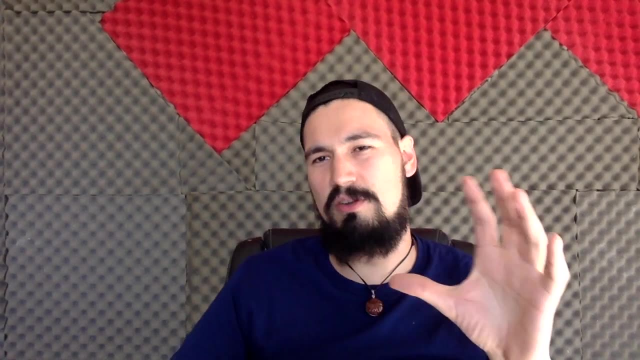 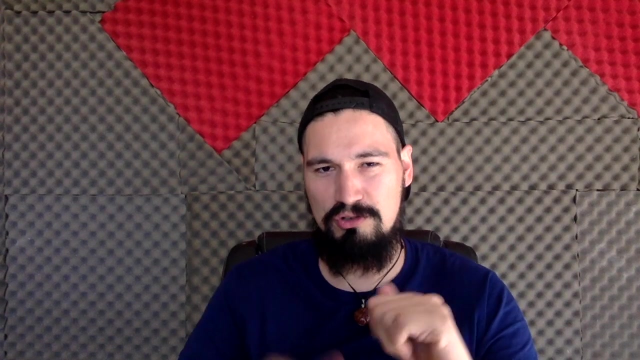 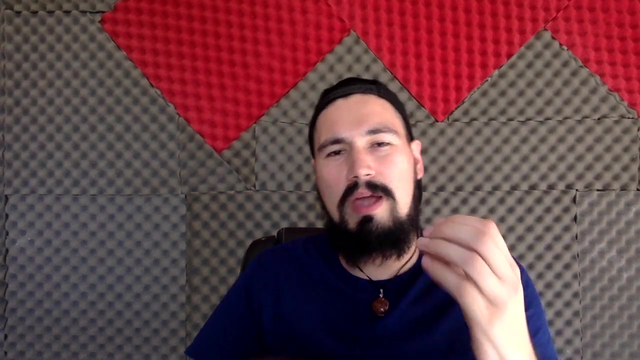 essentially for environment and for purification. okay, so how is the course structure? we're going to have first section, introduction. actually, what is the course about? the details, all that boring part? important because we need to understand how the course is structured. then, section number two: we start with a mass transfer review. what we want here is to get 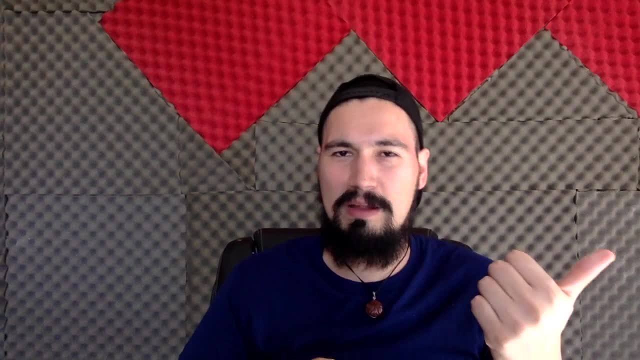 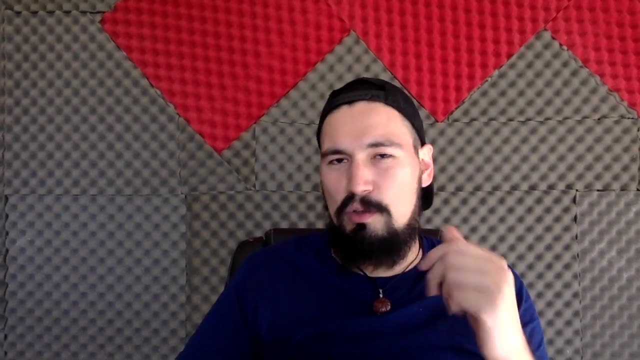 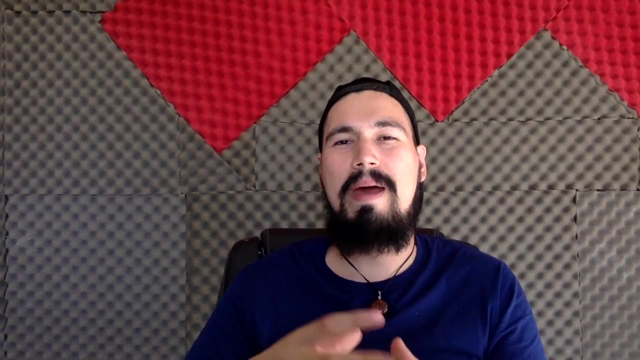 to know the importance of equilibriums. which laws are we going to use? henry's law, raul's law, how to apply them? vapor pressure, gas solubility. and once we get these very basic concepts, we start starting our course on mass transfer. what is diffusion? what is convection? 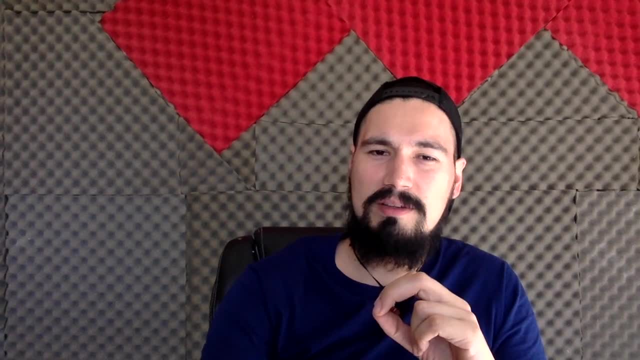 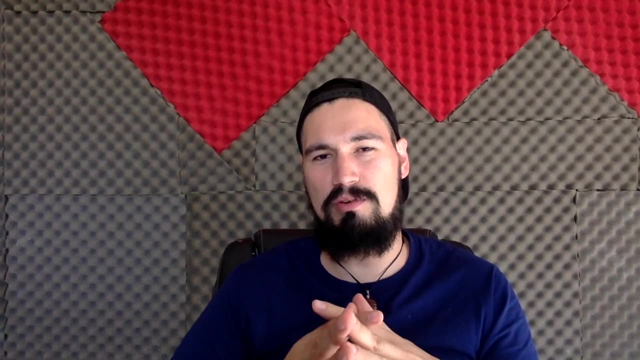 how can we model them? why are they required in this course? and then we continue to one of the most important theories, which is interface mass transfer. so interface, as the name implies, is between two interfaces. the first one is the interface mass transfer and the second one is 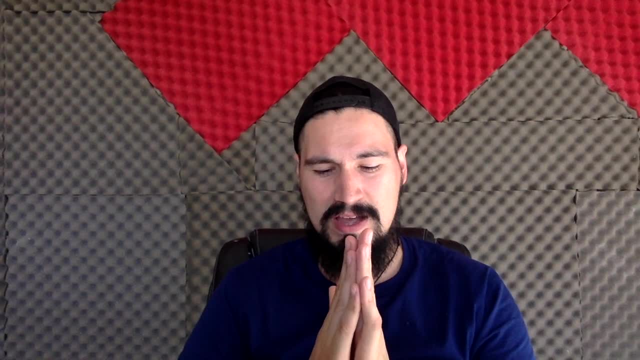 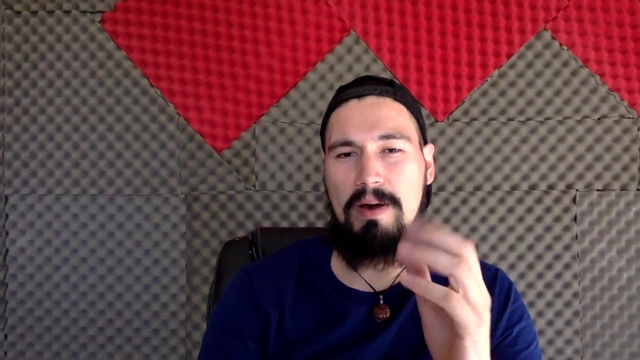 the interphase mass transfer. so interphase, as the name implies, is between two interfaces. interphase, as the name implies, is between two interfaces. we have the gas interface, liquid interface, and the idea is to make interaction through all the surface. then we start about talking about the two film theory, how to model it, how to get mass. 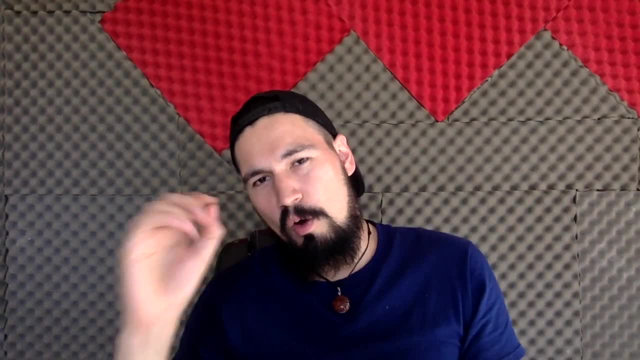 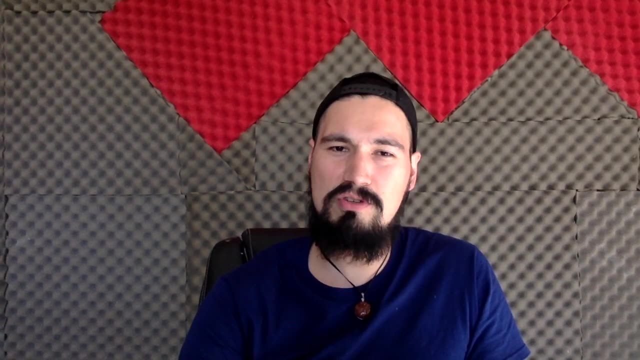 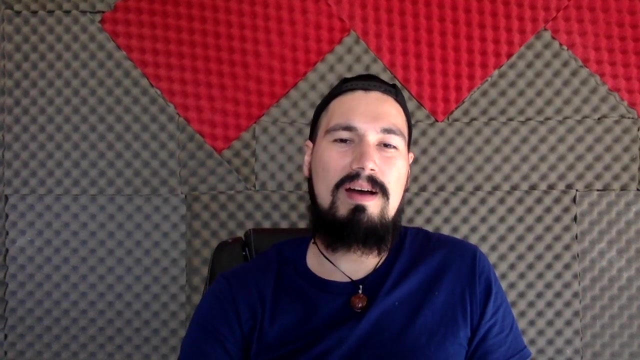 transfer coefficients, local mass transfer coefficients and overall mass transfer coefficients. once we get to know that we are ready to continue with section number three, gas absorption, we get to know what is this operation. why do we need it, why do we need to apply it? what are the main scope of the course? should we use only physical absorption, chemical? 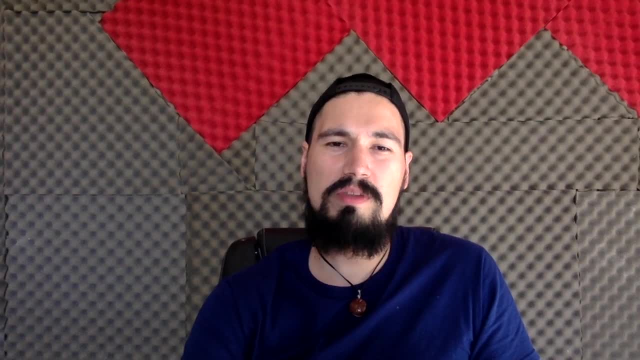 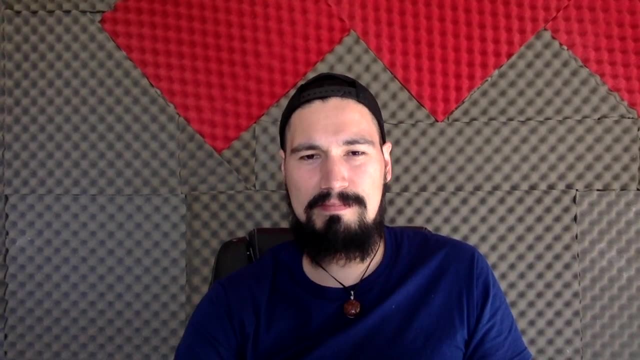 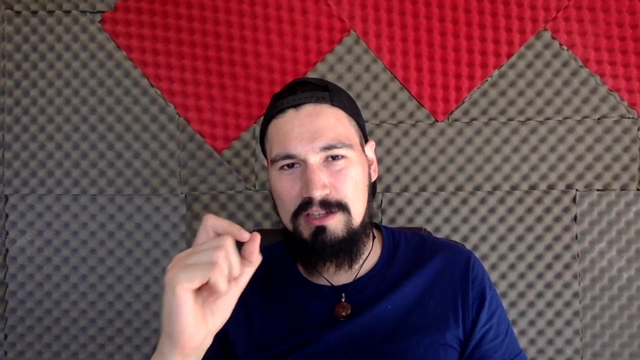 absorption and so on. then we get to know the four main types of gas absorption operations. we learn about the design steps, how to select a solvent. whatever application you're going to use in gas absorption, you need to know how to select the solvent. and then we get to our main operation. 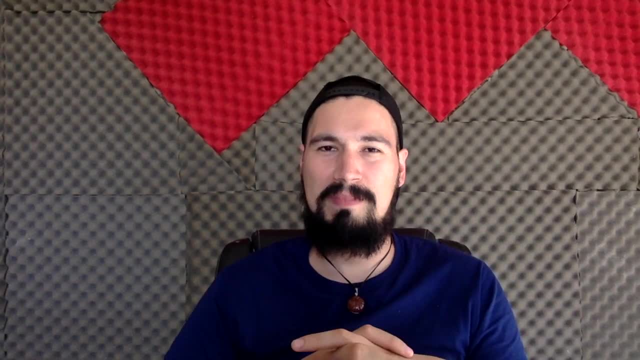 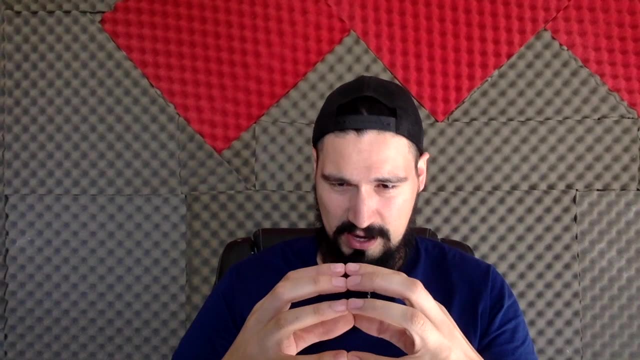 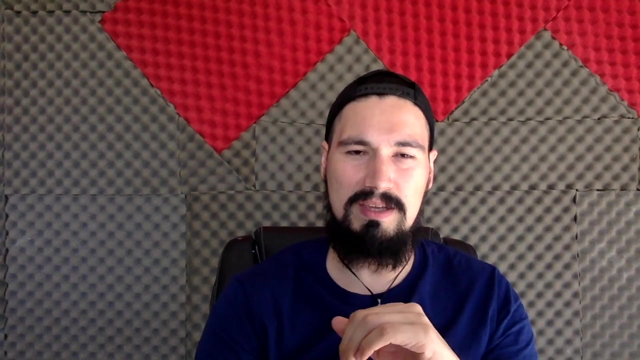 or main unit operation, which is tray columns. what is a tray column? as the name implies, we have several plates or trays in a column. we're going to see how equilibrium is interacting in these stages. how many trays do we need in order to achieve the interactions? what are the sieve trays? valve trays? 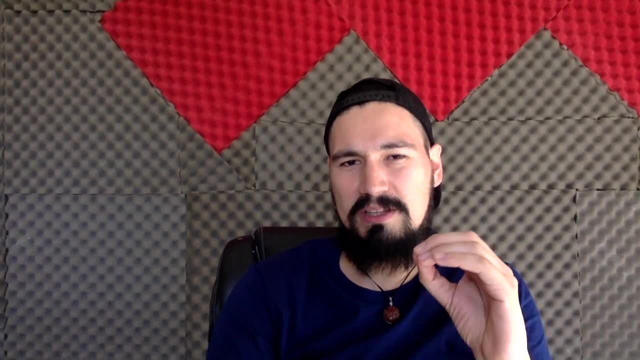 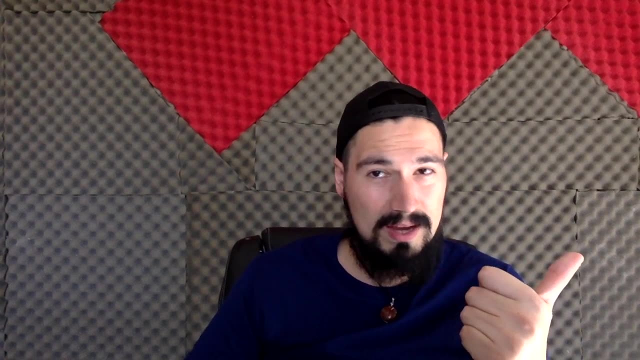 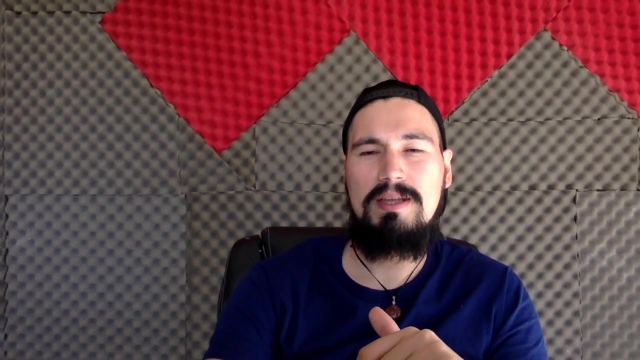 bubble cap, trays and so on. all the column internals are also considered there, and then eventually we need to get to the mat. so we're going to see that what's the operation line, the equilibrium line, how to select the total number of stages, what is the minimum solvent flow rate, co-current flow counter, current stripping, absorption and so on. then we get. 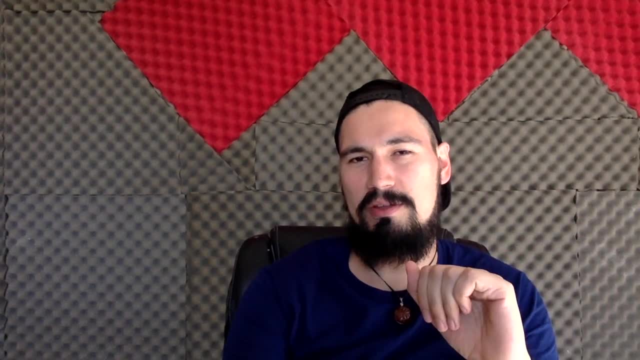 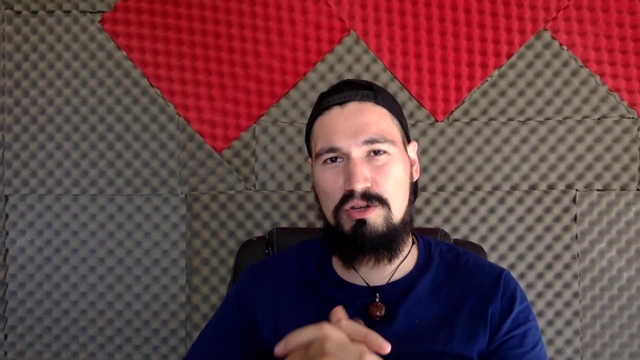 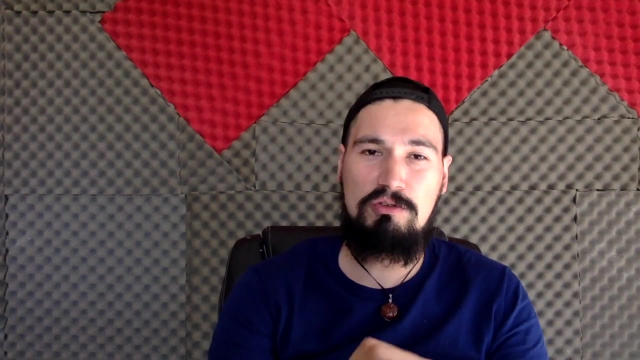 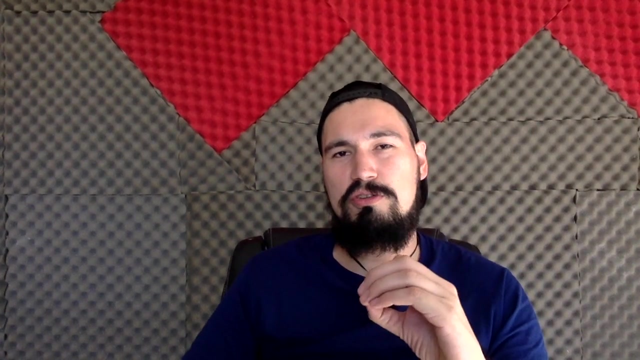 also not only the graphical method but the analytical method for total number of stages. then we continue with another important unit operation which is packed columns. so in the packed columns, at the name implies we need to fill it with packings. we're going to learn about packings. what are they, what are their properties, the materials requirements, etc. we also see the 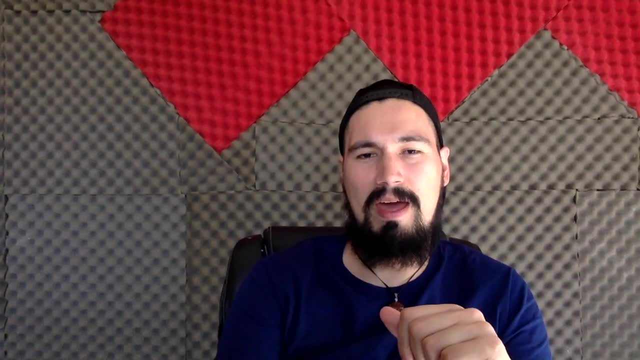 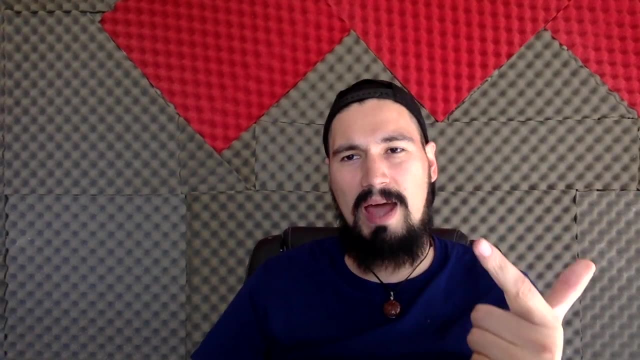 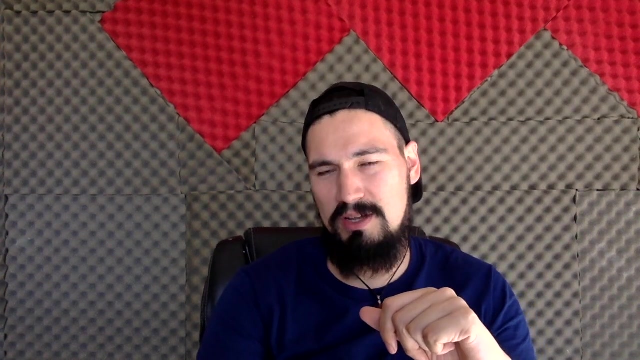 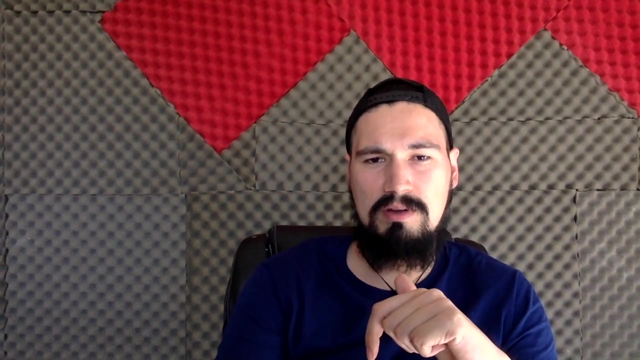 different column internals required for packings and once we get more into the design and model, we're going to see that this is based on column diameter, total height, the height equivalent trace for the packings. also, we talk about the mass transfer units. thedon't celebrating Александri, just wanted to say THC-arr. it's still disadvantage to 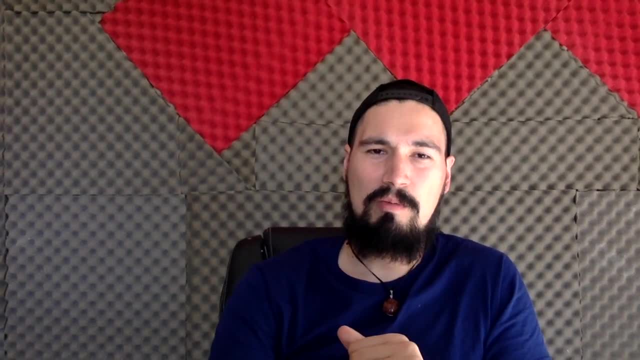 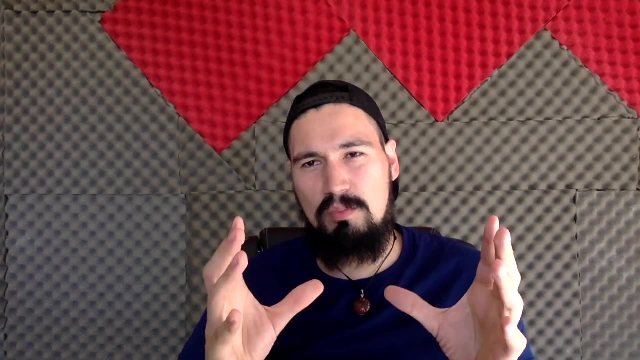 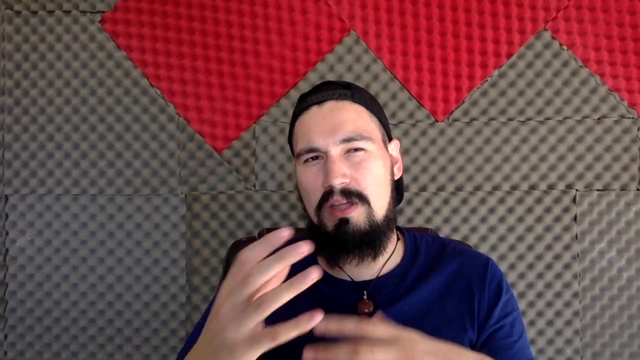 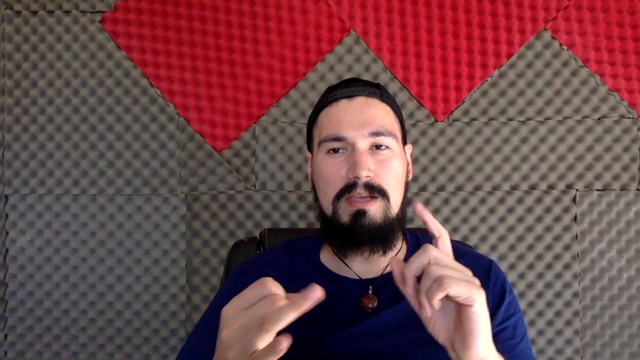 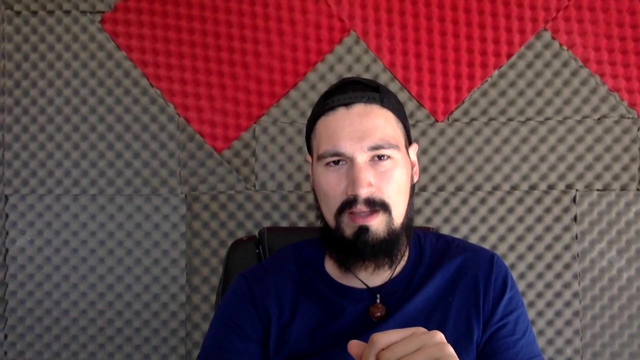 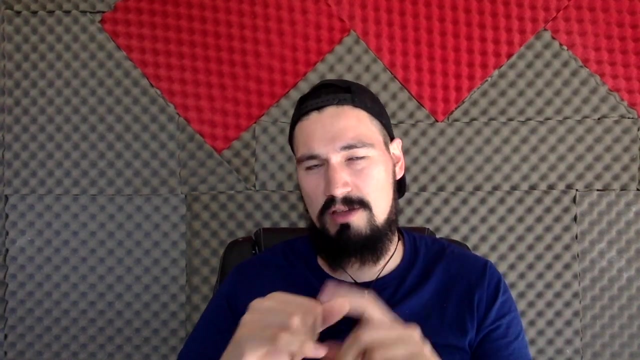 measure the quality of lectern sek toda in. so in this slide we model maybe a non-diluted case, a multi-component absorption case or an absorption with chemical reaction. Then we finish with a set of simulations, If you have a process simulator, for instance Aspen Plus, Aspen, HiSys or maybe 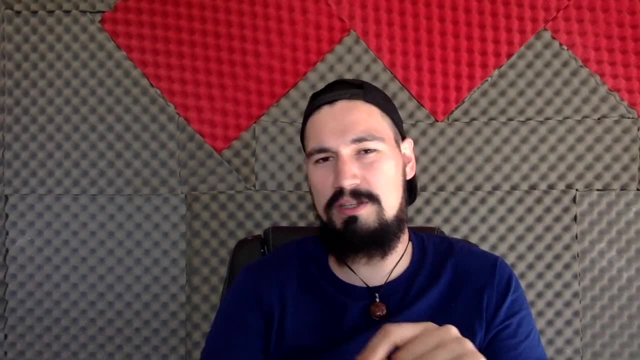 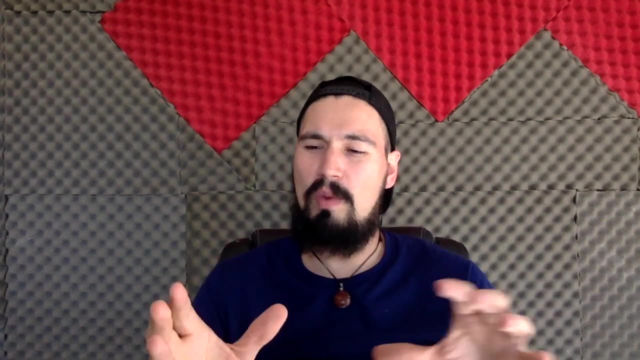 Pro2, or ChemSys, CoCo, etc. This is very enriching for the course because we're going to see simulations. we're going to see what-if scenarios. what happens if we increase the flow rate? what happens if we decrease the composition here? what?